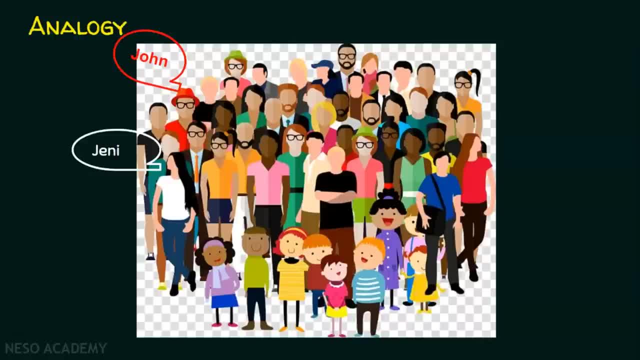 Now answer this question In this group. if John and Jenny are talking to each other, will others hear this conversation? Think of this question and the answer is yes. Those who are in the coverage range of John and Jenny can hear the conversation, because John and Jenny are not the only participants in the group. 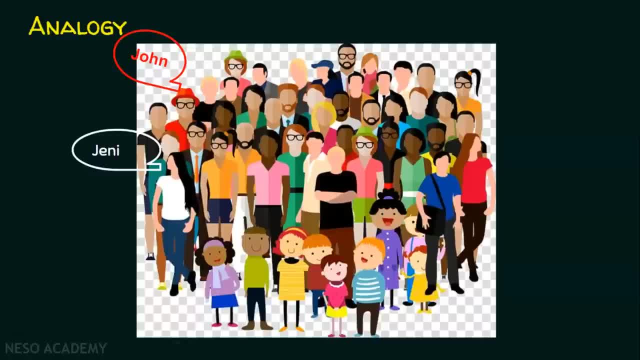 Though others are also in the coverage range of John and Jenny. others can hear the speech signals of John and Jenny, but they normally ignore this conversation because these conversations are not intended to them. Now, this analogy is related to computer network. In computer network we have wired network and we have wireless network. 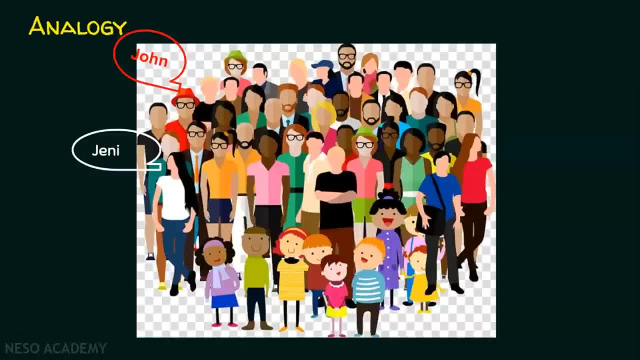 In a wired network we can do unicasting so that the signals from the sender can be received by the receiver When the signal is transmitted over wire- it is not giving room for others to know this conversation- But in wireless, in a coverage area, if a sender sends the data. 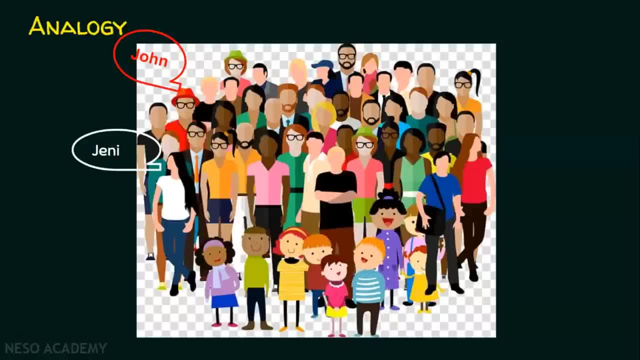 whoever is in the coverage area of the sender, they can still hear the conversation. So in wireless, this is one of the major areas of security concern. Now let's dive into the topic. The topic of the session is IEEE 802.11. 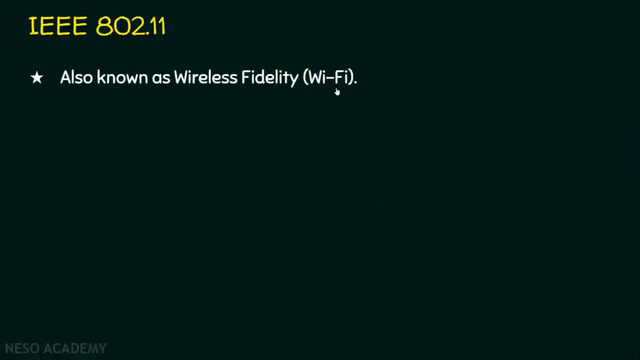 It is also known as wireless fidelity, which is known as Wi-Fi, And, like its Ethernet and token ring siblings, these two are wired LAN technologies. IEEE 802.11 is designed for a use in a limited geographical area, maybe in homes or in office buildings or in public spaces. 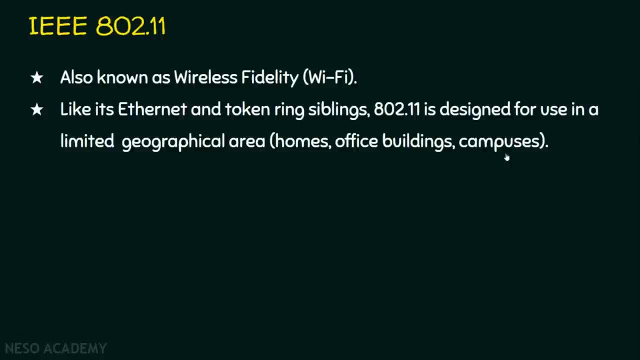 IEEE 802.11 is designed for a use in a limited geographical area, maybe in homes or in office buildings or in public spaces. So IEEE 802.11 is a wireless LAN technology And the primary challenge is to mediate access to a shared communication medium. 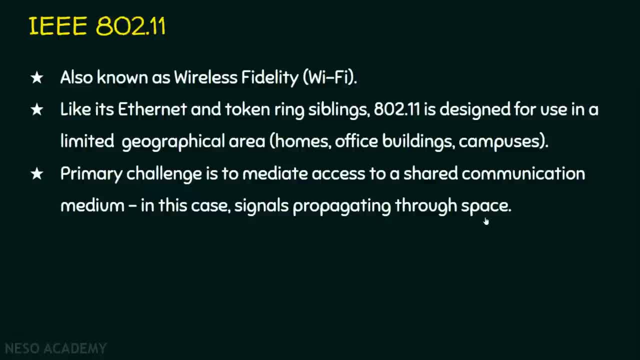 In this case the signals propagating through space or air. That is what we have seen in the analogy. Always there is a security concern with wireless, And we know IEEE 802.11 Wi-Fi is mainly for wireless LAN. In addition to this, 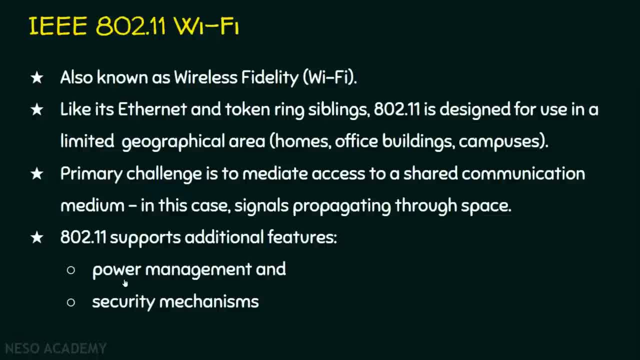 this 802.11 supports wireless LAN. In addition to this, this 802.11 supports wireless LAN. In addition to this, this 802.11 supports wireless LAN. They are power management and the security mechanism. Now let's see an example. 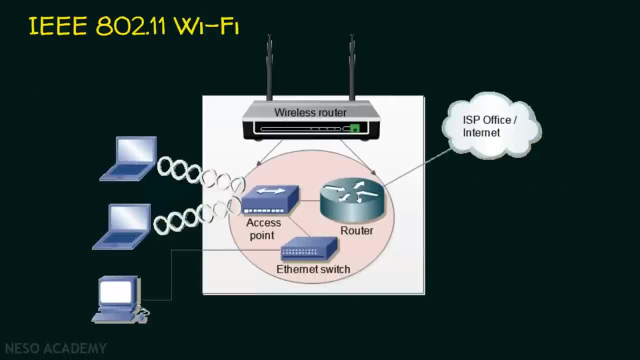 In this example we have a router. This actual router is connected to the ISP, that is the Internet Service Provider's office, And we get internet connectivity from this office to our campus network. Let's say this is our router, which is placed in our campus. 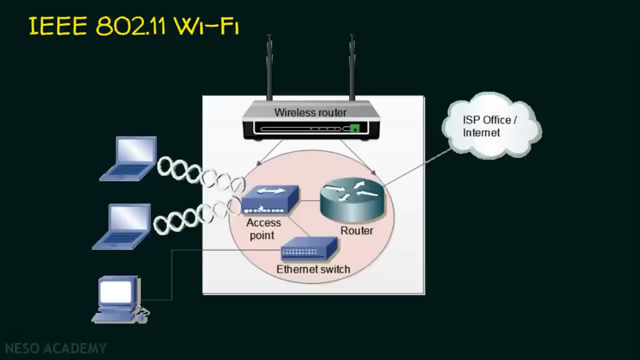 Now, with this router, is connected to the wireless access point. Let's say, this is the Wi-Fi access point where many devices can connect to it. So we can connect to this Wi-Fi access point Not only laptops, we can also have mobile phones. 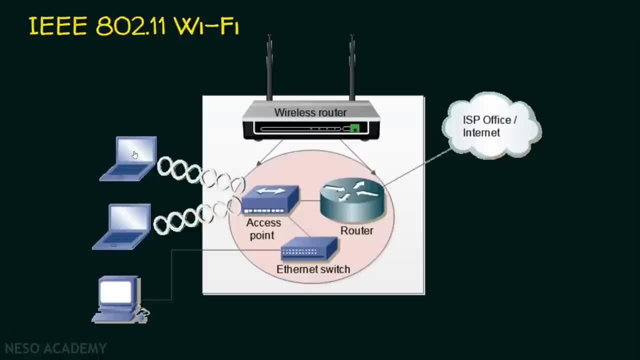 Now what happens when this computer wants to connect to the local area network, So it gets connected to the wireless access point first, In turn, if it wants connectivity with its local area network so it can participate through this Ethernet switch where there are many devices connected with this Ethernet switch. 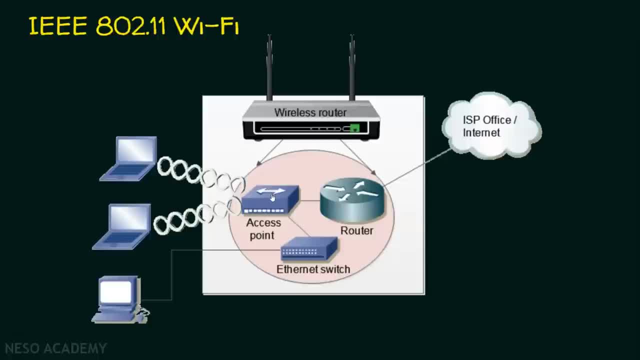 So from this place to this place it's wireless, And from this place to this place it's a wired technology, So protocols will take care of these activities. Now in case, if this client wants internet connectivity, let's assume there is a user who is working in this laptop. 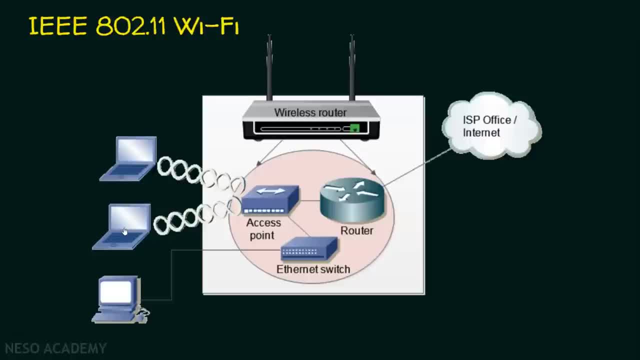 who wants to access googlecom How we will get googlecom connectivity. He opens a browser and the connectivity between these two is 802.11, that is Wi-Fi technology. So between this access point and router, it is a wired technology. 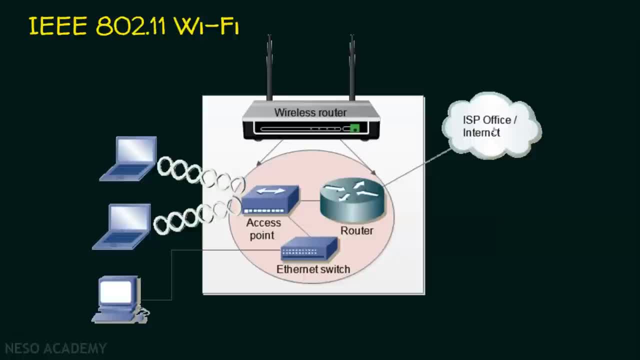 And it becomes the responsibility of this router to forward the packets to the ISP router And in turn we will get internet connectivity. So this router can also be replaced with the help of a wireless router. In this case we have a wireless access point. 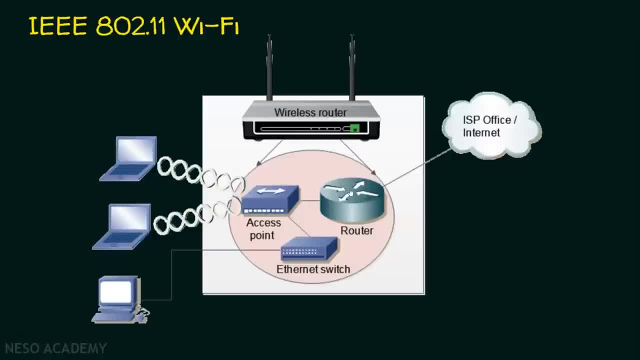 and we have a router which works with wired environment only. If you observe, both the interfaces are wired interfaces only. We also have an access point which is connected to the Ethernet switch, So we can also replace this entire thing with a wireless router. 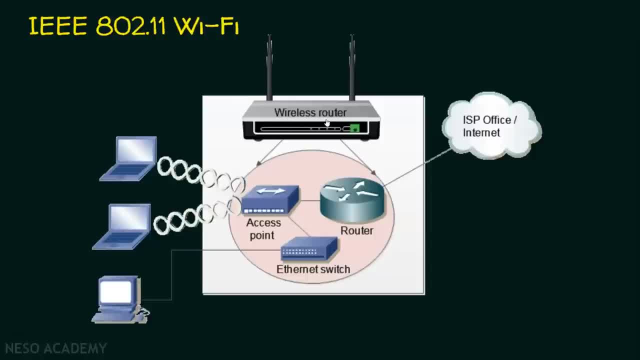 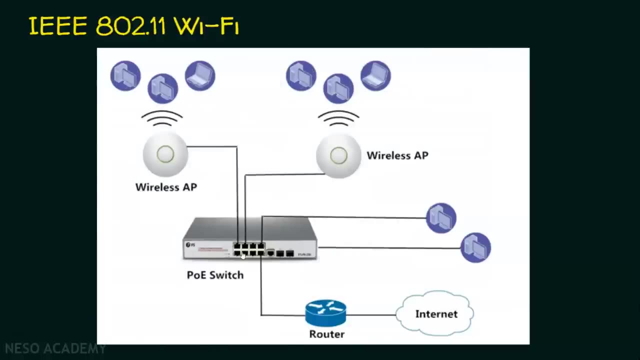 where this wireless router provides the functionality of a router, but with the help of wireless technologies Also, it can extend its capability by providing one of its interfaces to establish a local area network also. Let's see one more example. Say: in this example we have a switch. 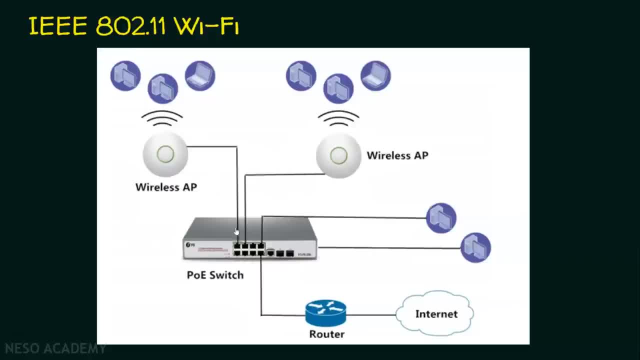 This switch is providing connectivity to two wireless access points- Let's assume this is wireless access point one and this is wireless access point two- And these two wireless access points are connected to this Ethernet switch. Now, if you observe, this is PoE switch, that is, power over Ethernet. 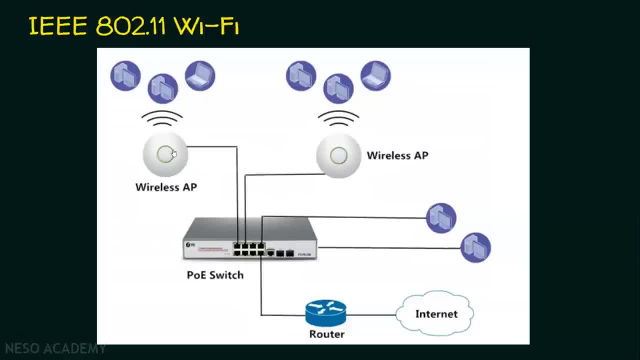 It means these wireless access points need not have a separate power supply. The Ethernet cable which is connected between this switch and this wireless access point will also carry power- And this is what we call as power over Ethernet- And, for example, if this device wants internet connectivity. 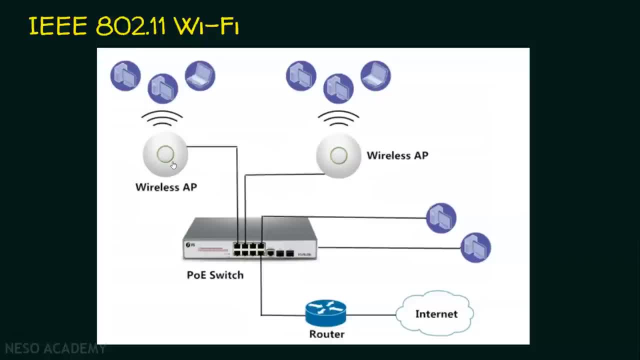 how this device gets internet connectivity. It is connected to the wireless access point. This wireless access point in turn is connected to the switch, and this switch is somehow connected with the router. Now this router forwards the data packets to the internet. So here we have a wireless LAN. 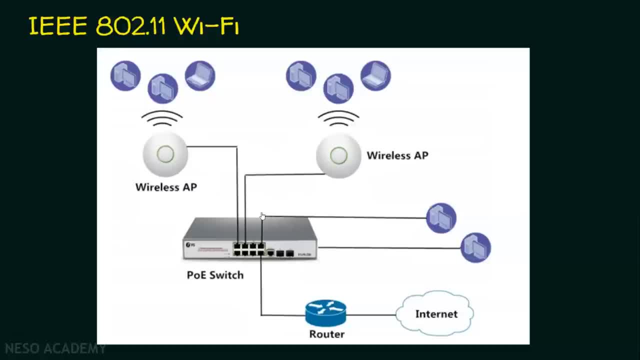 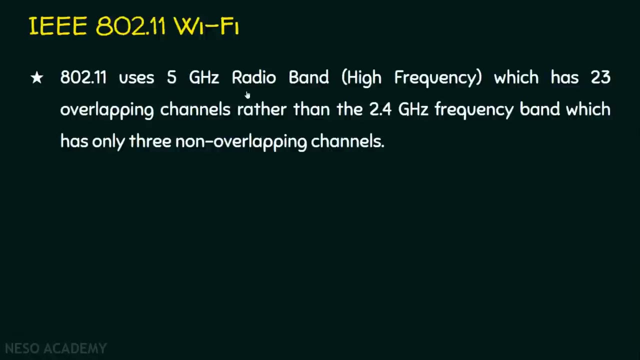 and here we have wired LAN, Because these devices are connected to the switch with the help of wires, Whereas these devices are connected to this network with the help of wireless. Let's now see more on IEEE 802.11.. This 802.11 uses 5 GHz radio band. 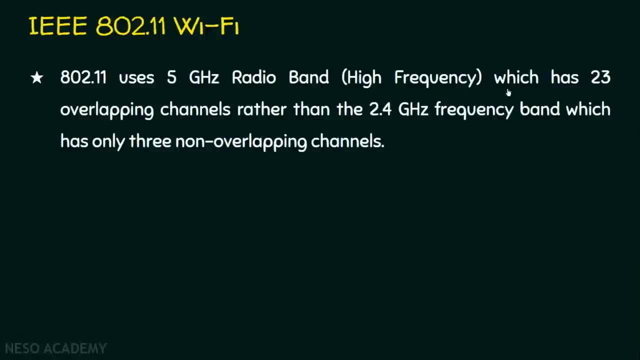 So it is a high frequency radio band which has 23 overlapping channels, rather than 2.4 GHz frequency band which has only three non-overlapping channels. IEEE 802.11 uses 5 GHz radio frequencies. Even it can work at 2.4 GHz radio frequencies. 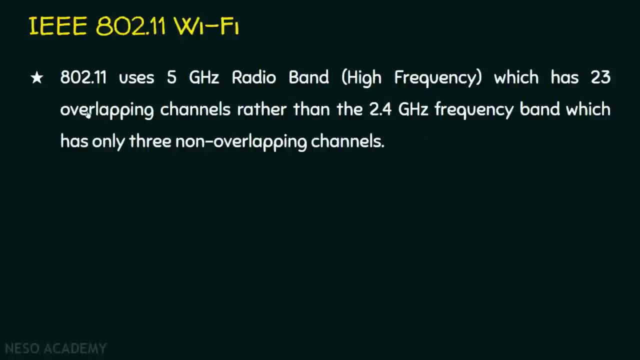 If it uses 5 GHz radio band frequency, it has 23 overlapping channels. If it can use 2.4 GHz frequency band, it has three non-overlapping channels. So, whatever the case is, we can use IEEE 802.11, that is, this WiFi technology. 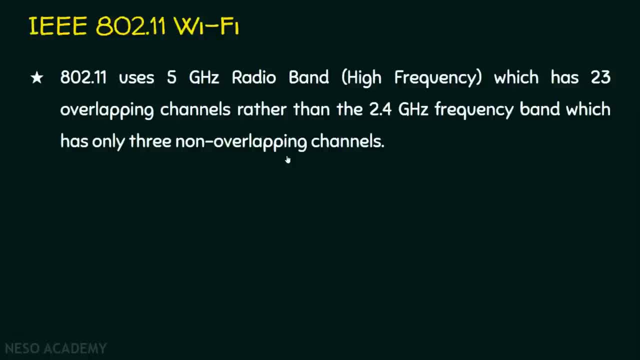 for our wireless local area network. Let's recollect what's the access point, What's the access method used by Ethernet, that is, the wired LAN. Ethernet uses CSMA-CD, that is, carrier sense, multiple access with collision detection. As I already mentioned, in wireless we cannot detect collision. 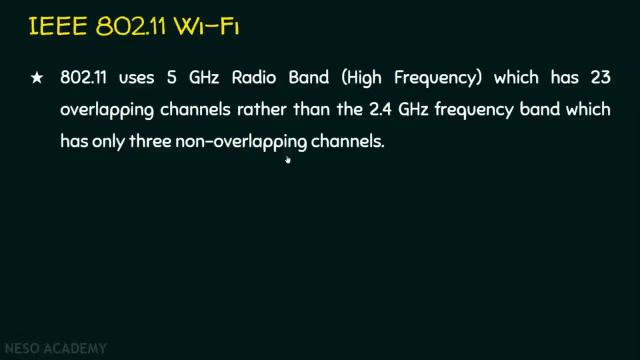 because the signals are propagated through air. So in WiFi, the access method of WiFi is CSMA-CA, which is carrier sense, multiple access with collision avoidance. Please make a note of this point. Ethernet uses CSMA-CD and WiFi uses CSMA-CA. 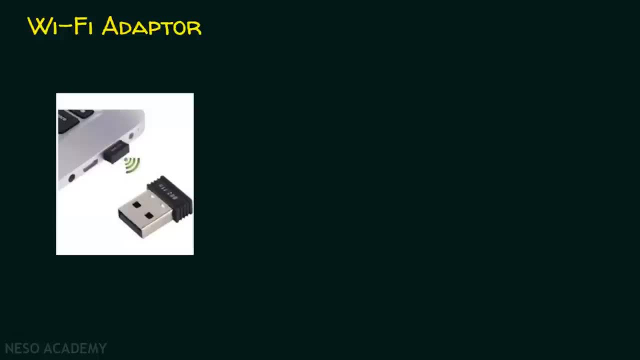 Now let's see the WiFi adapters. So we have WiFi adapters, which is very small in nature. In case, if we don't have a WiFi adapter to our desktop computer, also purchase this WiFi adapter. just plug this into your USB port of your computer. 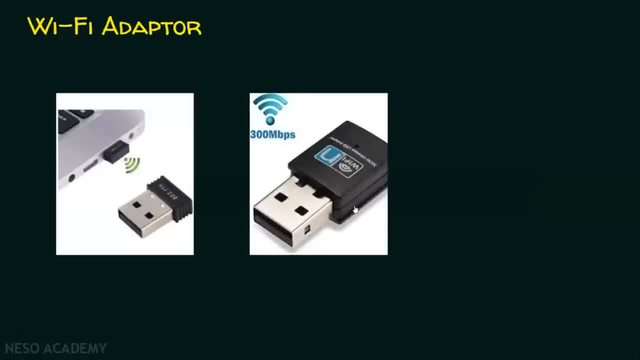 So we will get WiFi connectivity. We have WiFi adapter of this kind, we have WiFi adapter of this kind and this is the antennae. So far, we have dealt with WiFi and we have also seen the access method of WiFi. Now let's dive into the next topic. 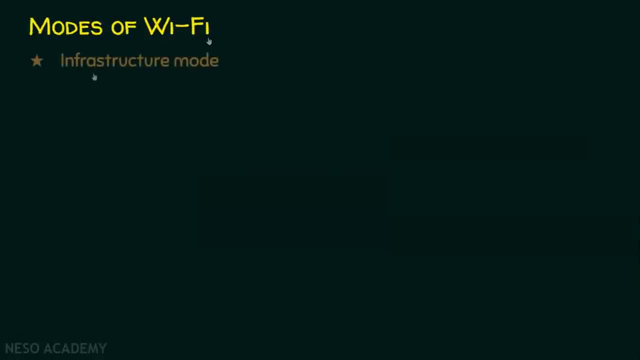 which is the modes of WiFi. WiFi, it works in two modes. Number one, it's the infrastructure mode. Let's see an example. Let's say: this is the wireless access point and this is the client machine that is connected to this wireless access point. 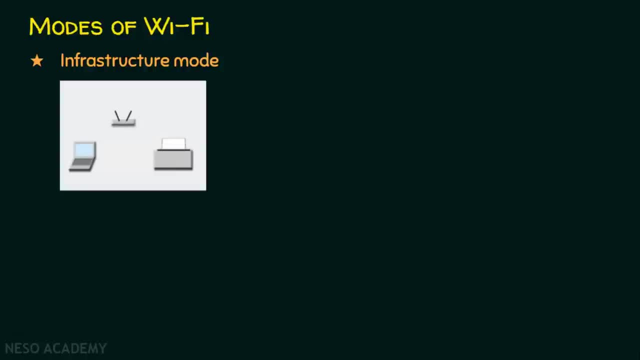 The client is sending the request for printout and the access point is giving that request to the printer. Now printer takes the printout. Now how this is done. It's not. these two devices are communicating directly. This is communicating with the access point. 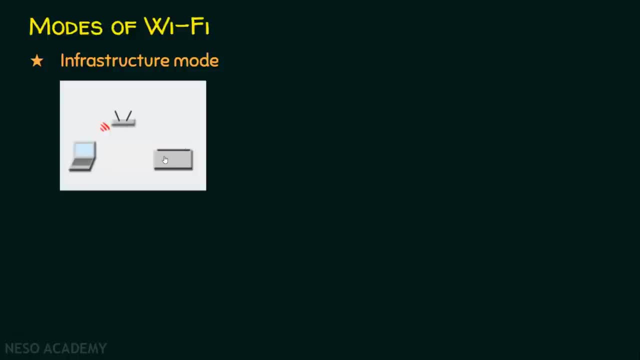 and the access point is then forwarding the data to the right device or the destination. Now here, if we have an access point and all the client machines are depending on the access point, which is also called as a wireless access point, We also have an ad hoc mode. 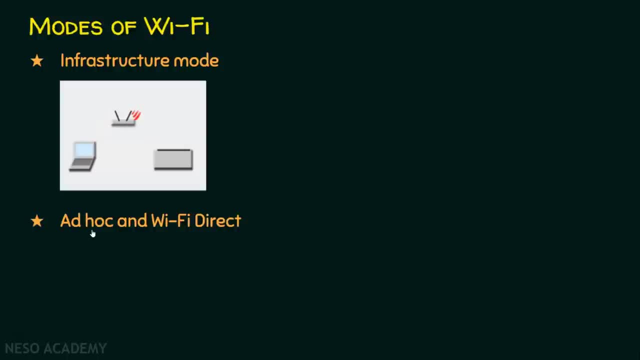 Ad hoc means we don't have any infrastructure. When we don't have any fixed infrastructure, then it is called as an ad hoc mode. In other words, infrastructure mode has a centralized administration, whereas ad hoc mode is decentralized. We will talk about this ad hoc mode and the infrastructure mode more in the next lecture. 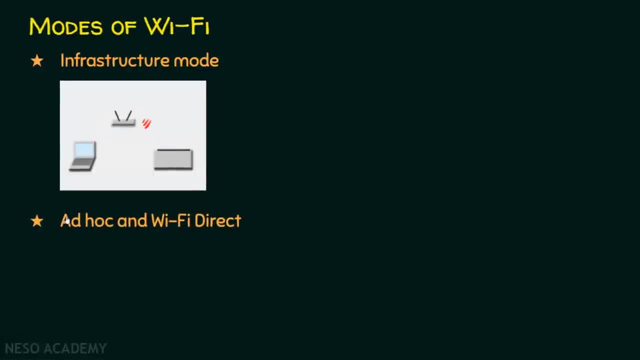 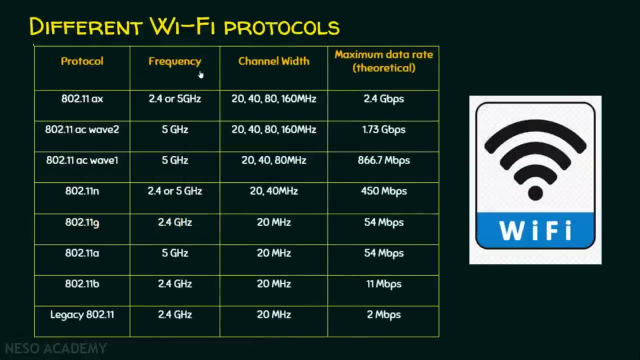 So Wi-Fi can work in infrastructure mode as well as in ad hoc mode. Before we conclude, we will see the different Wi-Fi protocols. Here is the protocol and we have a frequency, we have channel width and we have the maximum data rate.